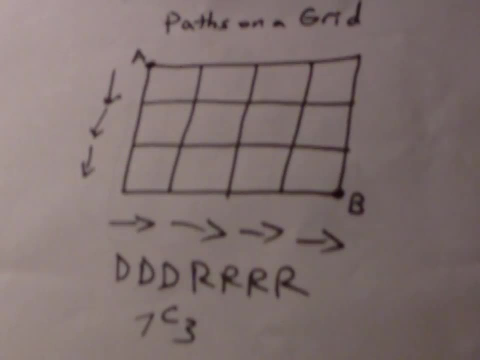 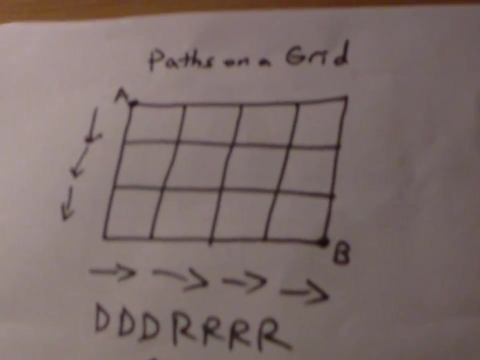 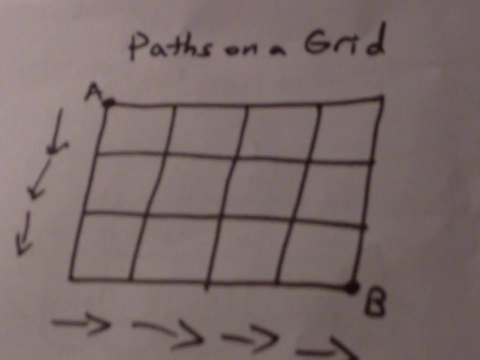 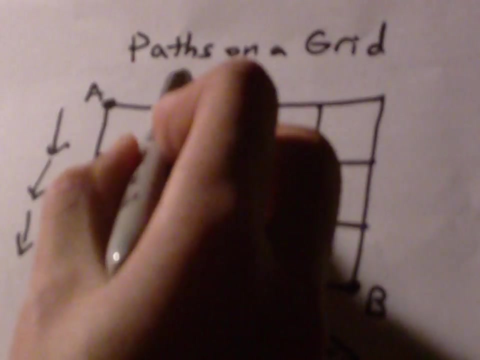 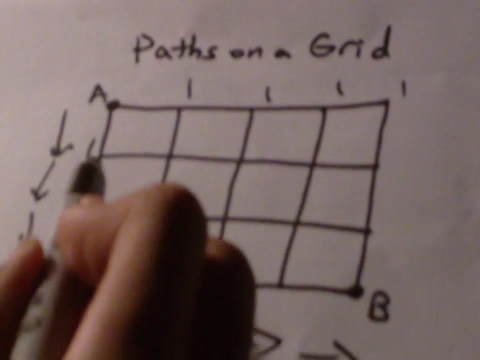 That would be 7C3, that equals 35. So the alternate way of doing this is not that useful for this kind of grid, because this kind of grid you can use something simple like this, but it's for more complicated grids. So to figure out how many ways you can get to point A, there's one way you can get to this point, one way you can get to this point, and so on. there's only one way to get to these points on the side. 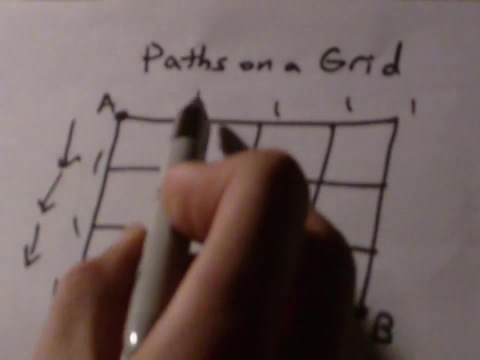 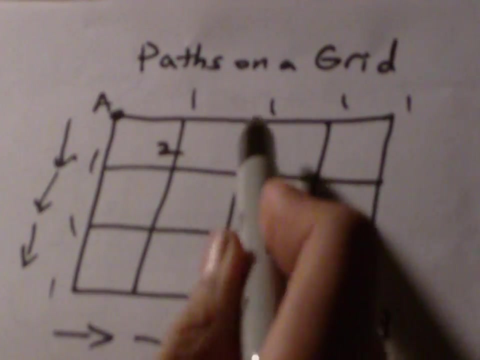 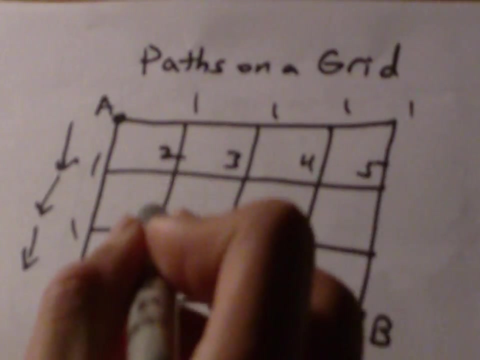 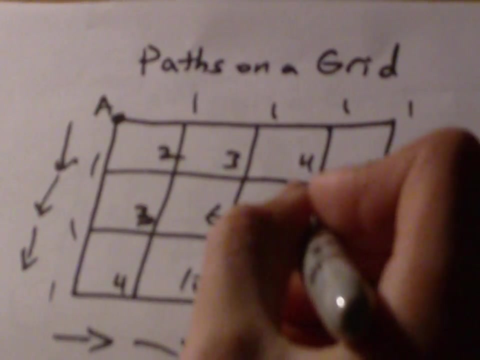 So then, how many ways can you get to this point? if you can get here one way, here one way, there's two ways, and so on, you can add the numbers at the intersections to provide this number. So we have 3, 4, 5, 3, 4, 6, 10, 10, 15, 20.. 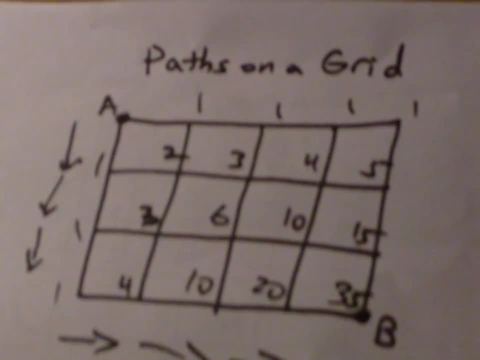 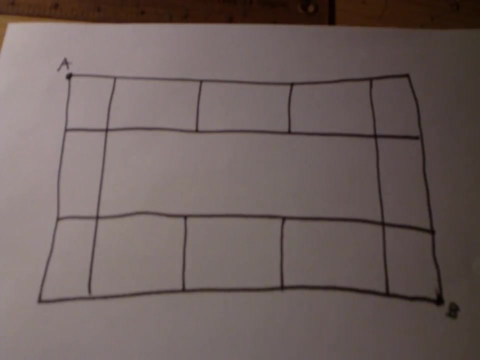 At the end, we end up with 35 as well. Now I'm going to show you an example of a way that this is useful. Okay, so here's an example. Here's an example of a grid in which you'll have to use the second method. 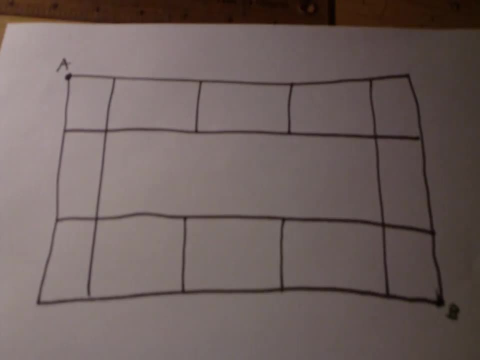 As you see, you can only go down and to the right in this grid. How many ways can you get from point A to point B? Well, using combinations here would not be smart because there's this big hole in the middle, So instead we use the second method. 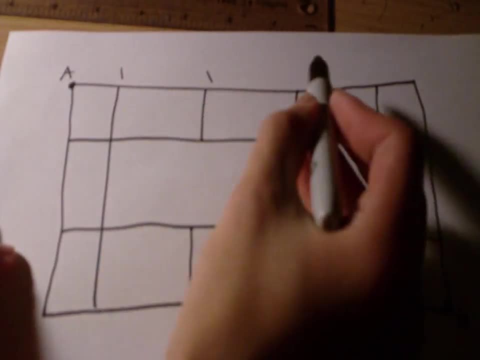 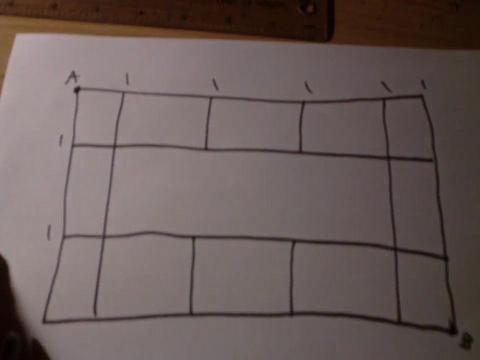 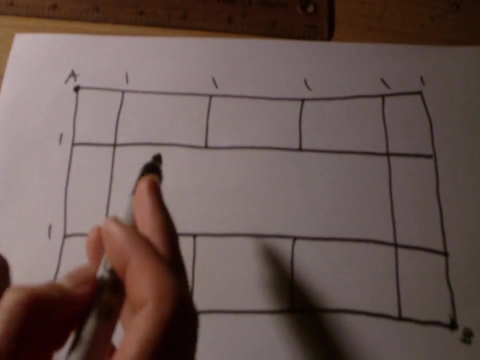 From A to here. there's one way, From A all the way along the side, as you can see, and from A down there's one way to get to each of these points. So to get to this point right here, we just have to add these two points. we get 2.. 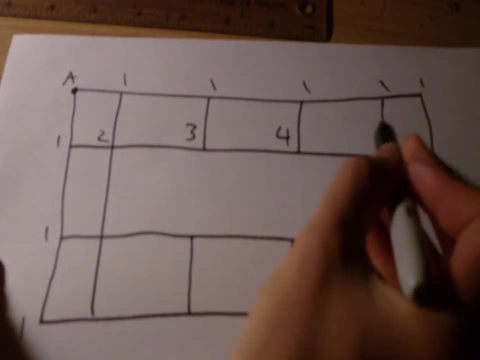 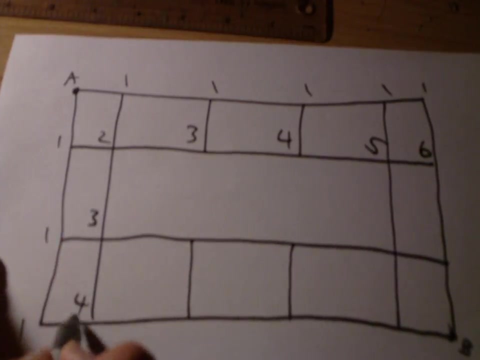 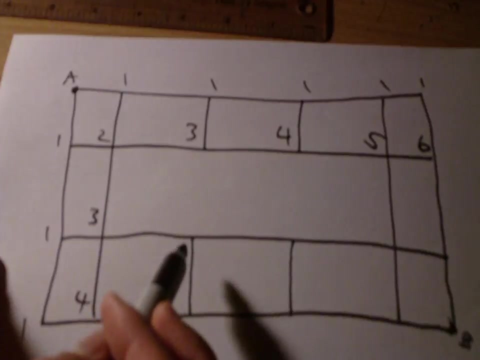 And so on. along this side we get 3,, 4,, 5, and 6.. And now, going down here, we get 3 and 4.. So a common mistake: you add these two, But there's no line right here in the middle, so we can't add.